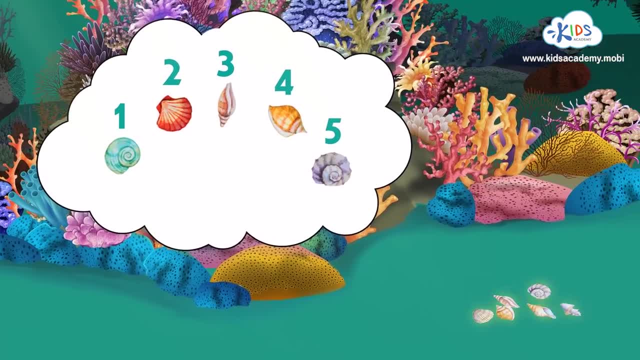 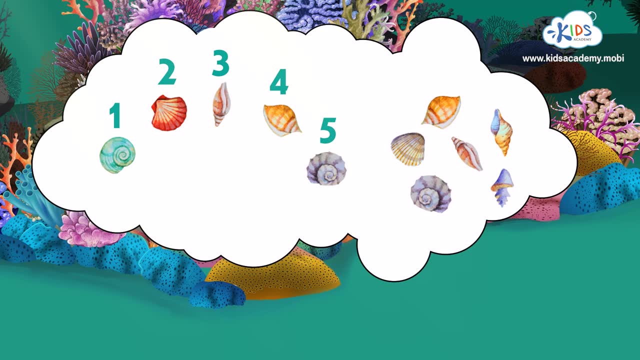 to make a necklace. See any more seashells. Right, there are 6 in the sand. How many shells have we got now? Well, let's see, We started with 5 and added 6 more. 1,, 2,. 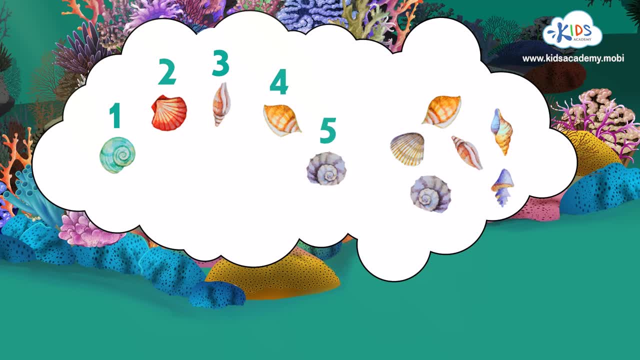 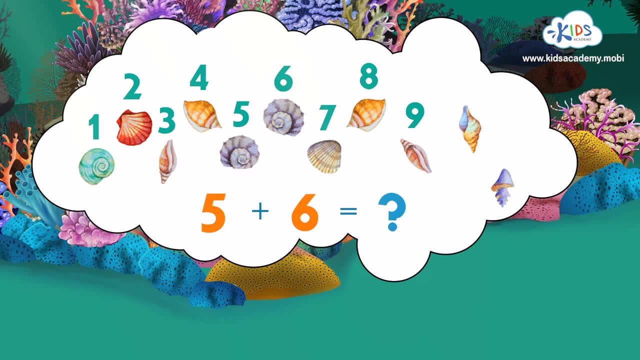 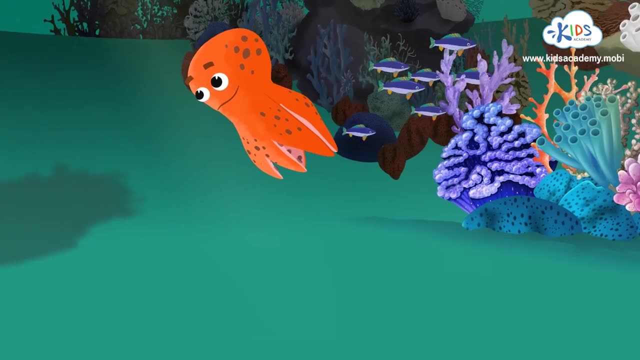 3,, 4,, 5, plus 6 more makes 6,, 7,, 8,, 9,, 10,, 11 seashells. in all, Let's go have a peek under that stone. Great, There are 4 seashells here. Let's add them all together, 11 plus. 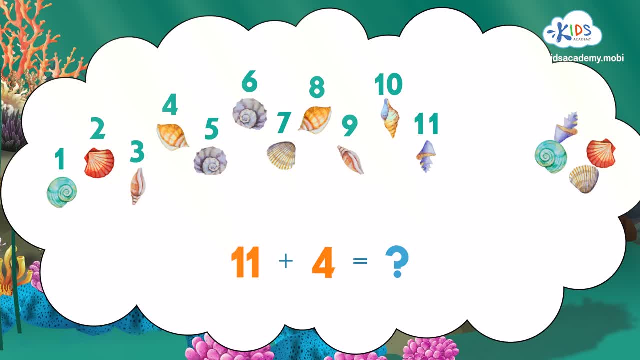 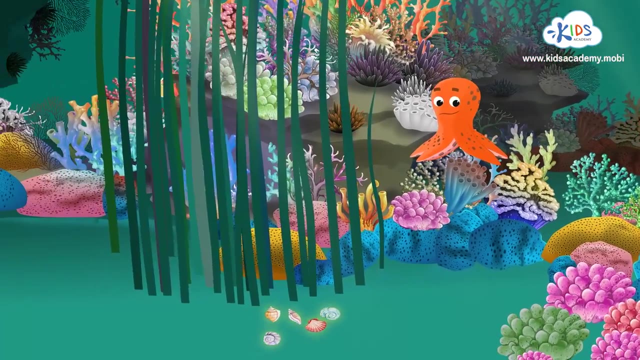 4 more makes how many seashells? 12,, 13,, 14,, 15.. So we've found 15 seashells so far. Good work. There are 5 more seashells near those seaweed strips. Now that we've found 5 more, how many seashells have we got in all 15. 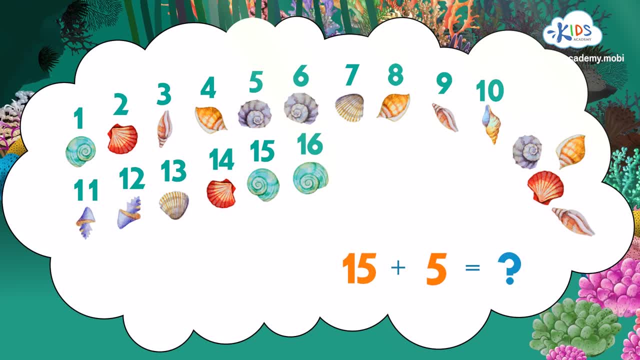 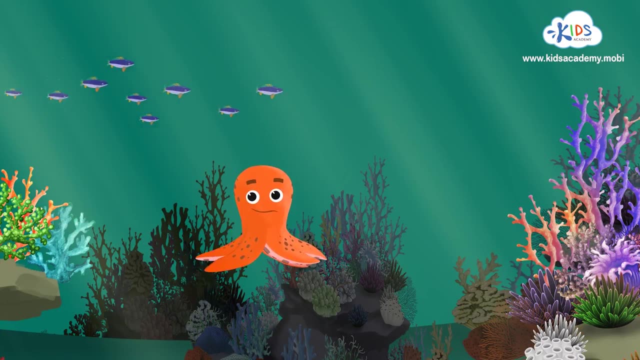 plus 5 more makes… 16,, 17,, 18,, 19,, 20 seashells in all. That's enough to make a beautiful necklace. Thanks for helping me find and count the seashells. Bye-bye. 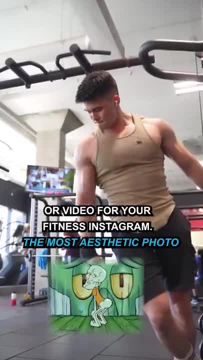 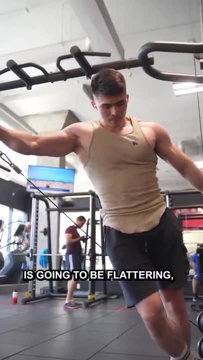 Here's how to take the most aesthetic photo or video for your fitness Instagram. Now it comes to Instagram and videos. people think they just need to be super fit, super jacked and any angle they're going to take is going to be flattering, right? No, Don't think like this, because it's an 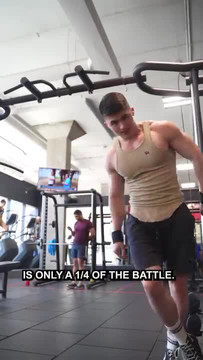 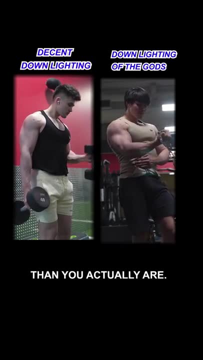 amateur mistake. In reality, a good body is only a quarter of the battle. So the very first obvious tip is take a video or picture under down lighting. This will make you look leaner than you actually are. Next, the angle of shooting or photography does matter as well. A wide lens will distort. 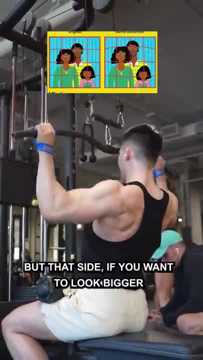 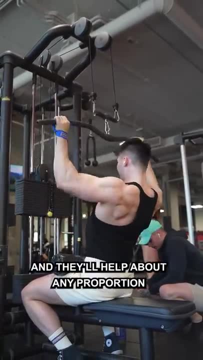 your body, such as an iPhone, a closer lens. But that aside, if you want to look bigger or make any other body part bigger, try shooting with that body part closer to the lens. That'll help balance any proportional problems. Now, lastly, always shoot from bottom to top so that it looks. 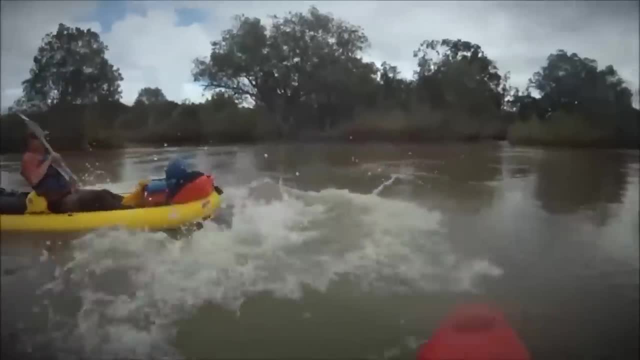 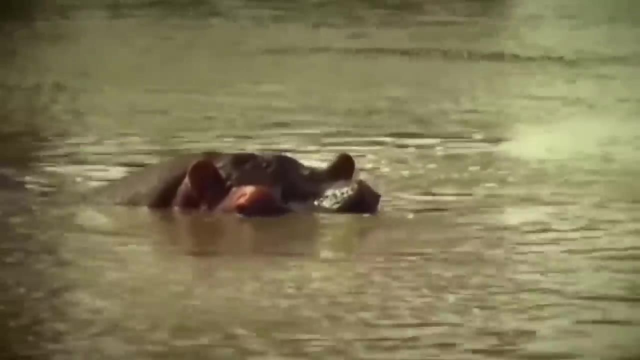 The following video features the deadliest real-life animal attacks covered on the channel thus far. These stories include the fatal mauling of their caretaker by a vicious pack of wolves, a man that was mauled by a hippo in front of his loved ones.